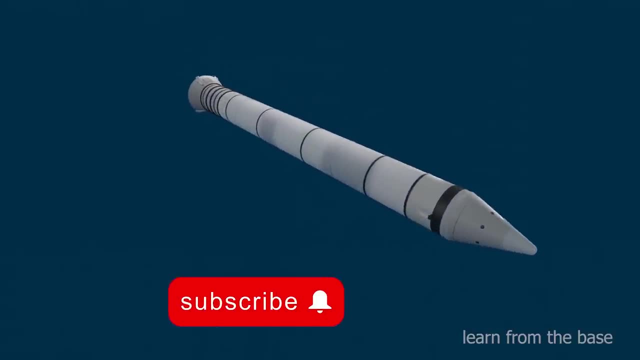 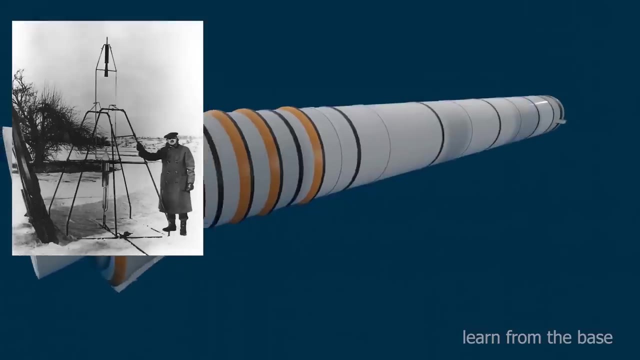 Rocket engines are one of the most difficult and complex machinery made by mankind. The first working liquid rocket engine was developed by an American scientist, Dr Robert Hutchings Goddard, in 1926. That rocket travel 45 feet during 2.5 second. 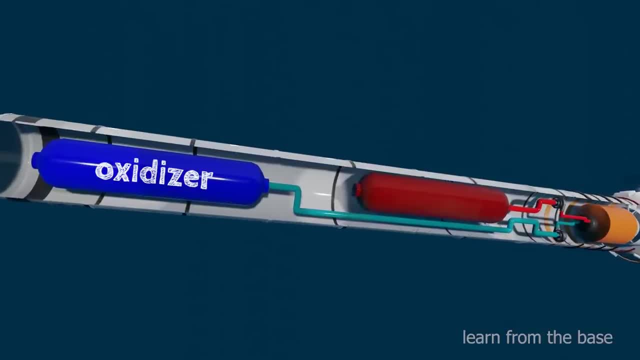 The rocket consists of two tanks. One is oxidizer tank and another one is fuel tank. The fuel and oxidizer are separately stored in these two tanks. they are in the form of liquid. The combination of the fuel and oxidizer are called propellant. 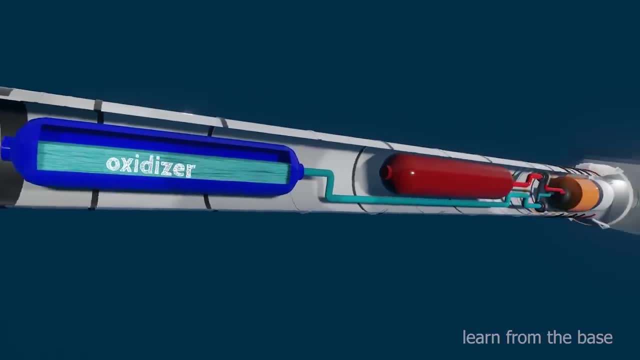 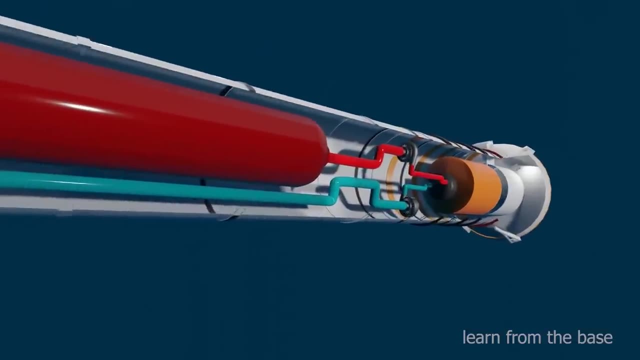 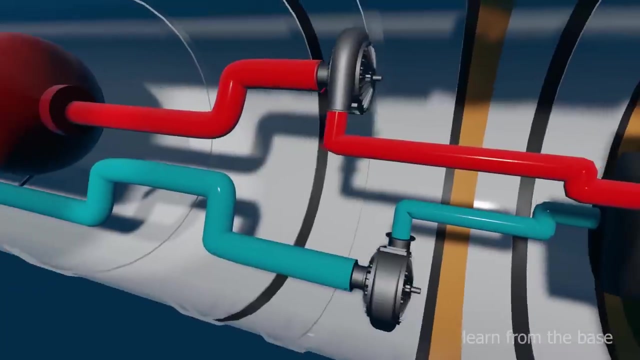 In liquid propellant rockets the fuel and oxidizer are in the form of liquids, so these rockets are called liquid propellant rockets, Couple of turbo pumps for pumping oxidizer and fuel tanks, are ordered by the company RMFCA which developed another rocket is RGkokzivets. 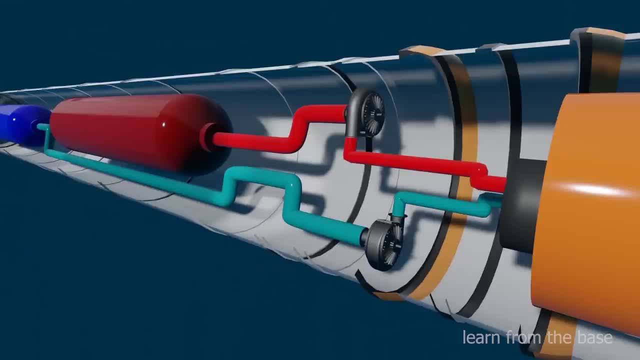 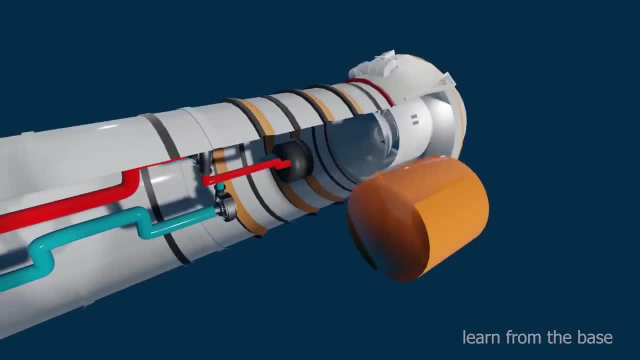 Yeah, I remember. some of them are made by myself. I think I need to make one too. The fuel and oxidizer tanks are in the form of liquid. These rockets are called liquid propellant rockets. fuel to the combustion chamber. Combustion chamber. 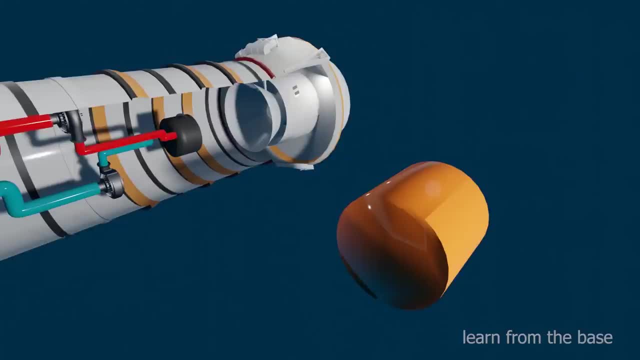 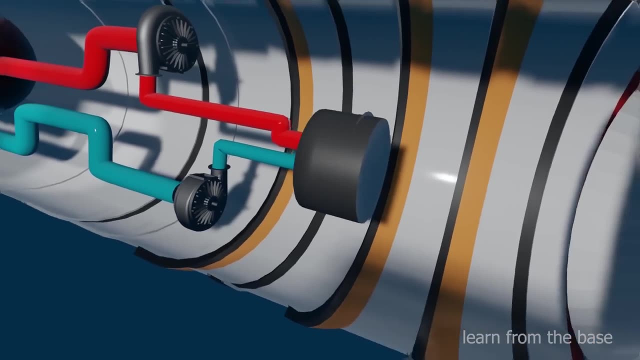 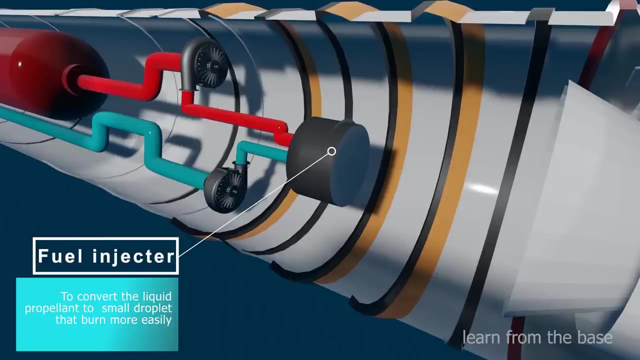 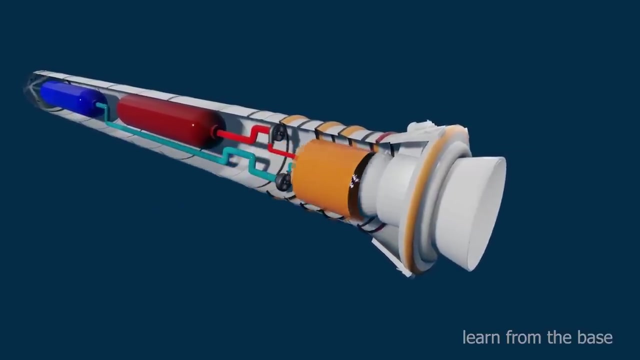 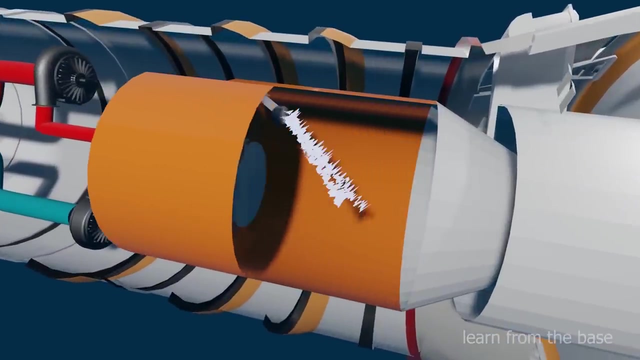 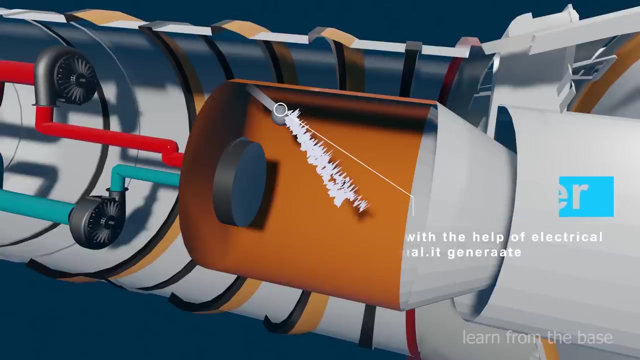 The fuel and oxidizer mixture are burning inside the combustion chamber Fuel injector. It convert liquid fuel and oxidizer mixture into small droplets and spray inside the combustion chamber Ignitor. With the help of electrical signal, it generates spark and burn the propellant. 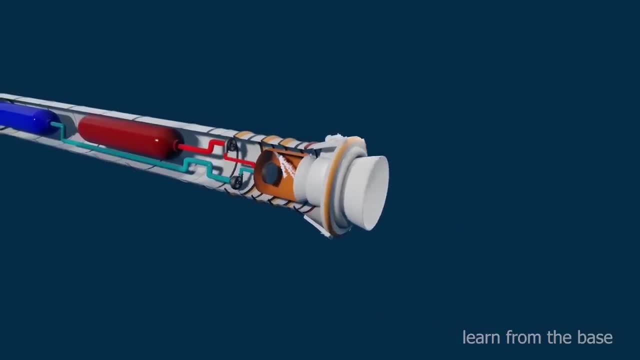 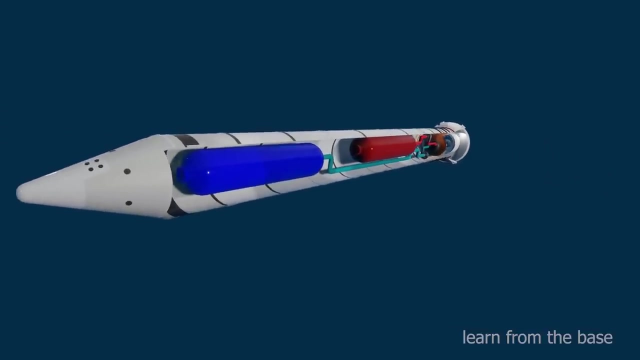 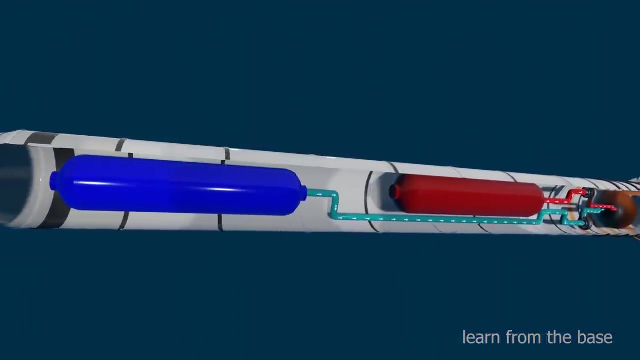 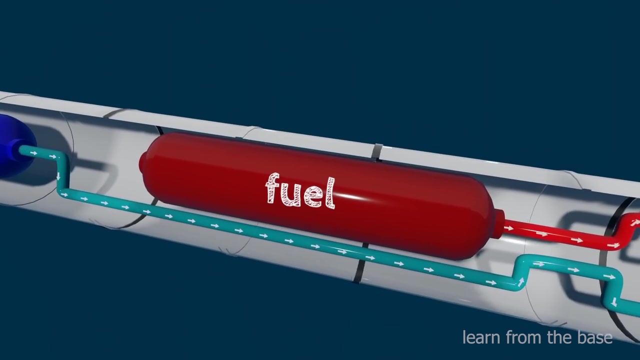 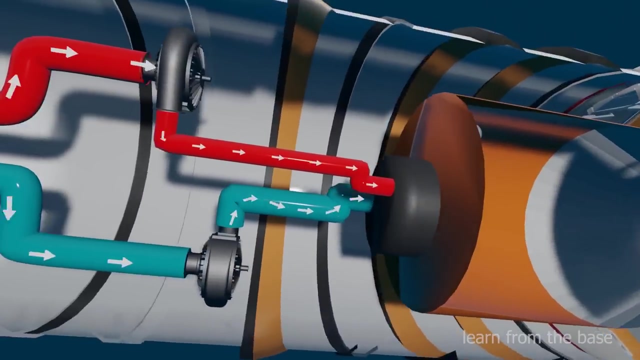 These are the nozzle That is used for expand and accelerate the combustion gas. Let's see the working principle of the rocket. With the help of turbo-pumps, the fuel and oxidizer are pumped into the injector. The injector convert the liquid propellant into.